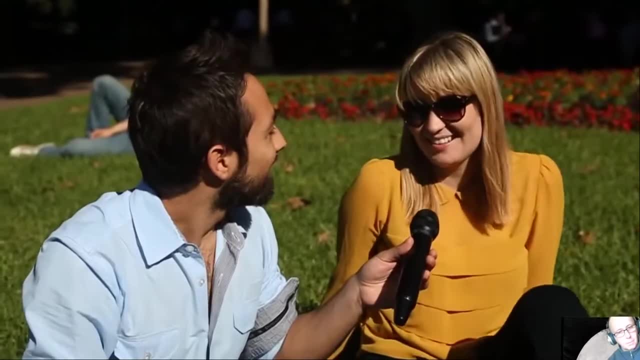 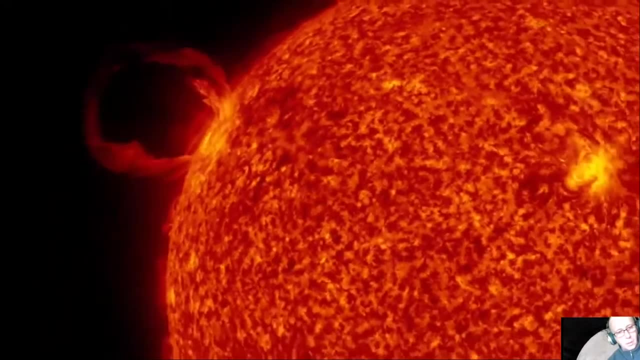 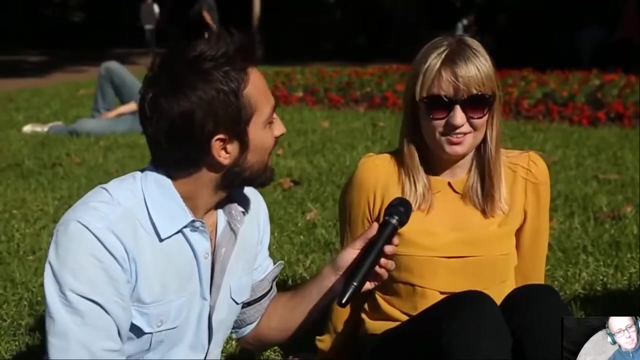 It's burning up Fire, The fire that's on the sun. But is the sun really a giant ball of fire? I mean, wouldn't it go out after five billion years? No, It's one of those things You just assume you know, but then you don't actually know. 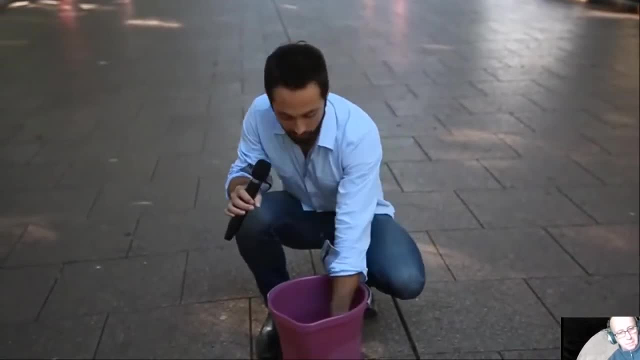 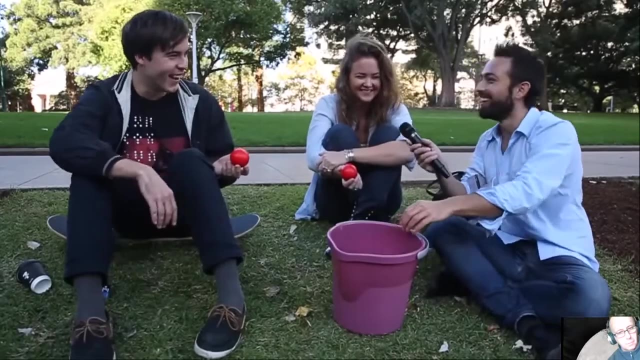 So in this bucket I have the components of the sun. Well, I have protons and neutrons. There are some electrons, but I didn't bring them Okay. Yeah, Most of the sun is actually protons, Okay. 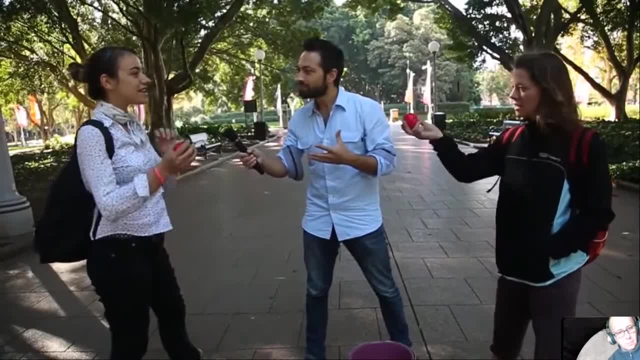 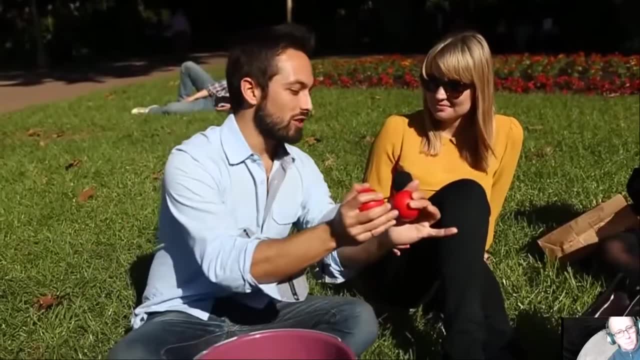 And so what do the protons do in the sun? It dance together, Okay, Okay. When they come close, you know what they do: They just Collide. Well, actually, they bounce off each other. I'm coming in. 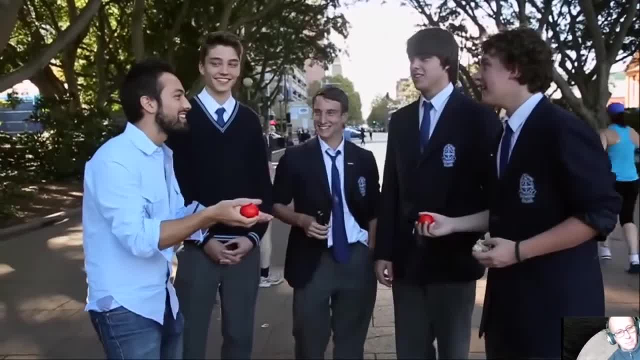 Whoa, Whoa, Whoa, Whoa, Whoa. Why do the protons bounce off each other? Something to do with electrons- Positive, negative electrons. Because they don't like each other. They don't like each other. 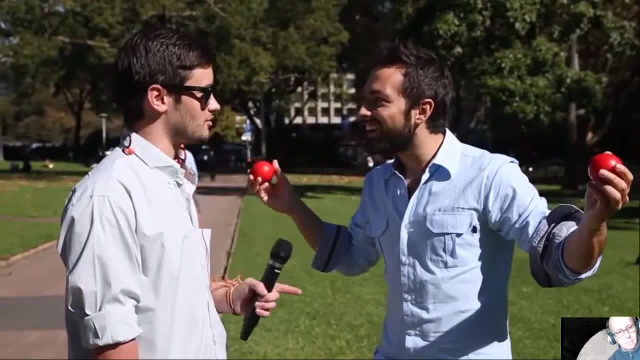 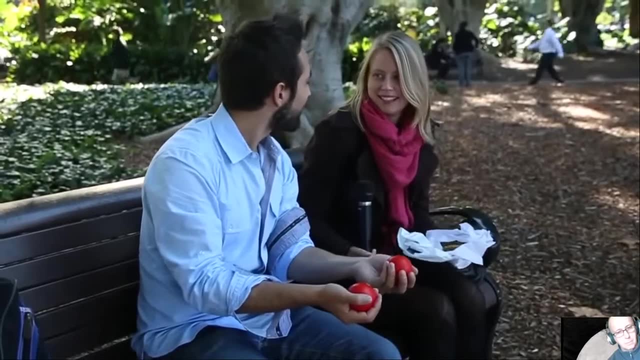 That's what it is. That's because a proton needs a neutron, right? Do you know why? they repel, like that Magnetic force, The repelling magnet type thing, Magnet field or Electric field. Positive and negative. Positive and negative. 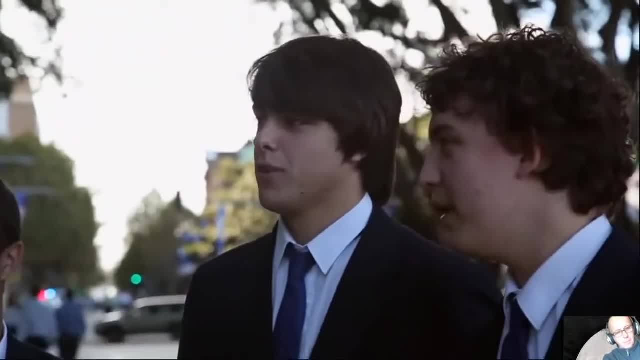 It's to do with the positive and negative, Positive and negative, Positive and negative. right, We got protons. Protons are Positive, Positive, Positive, Positively charged. Yeah, so the positives repel each other. Positive and negative charge. 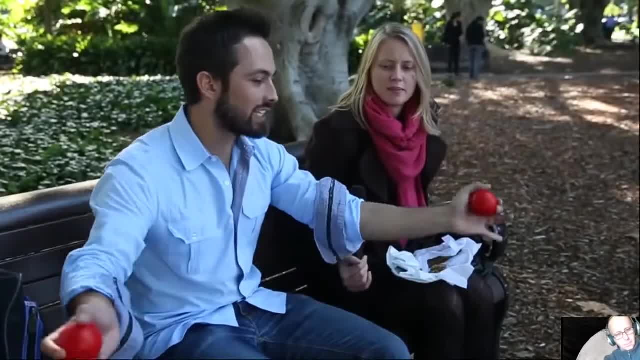 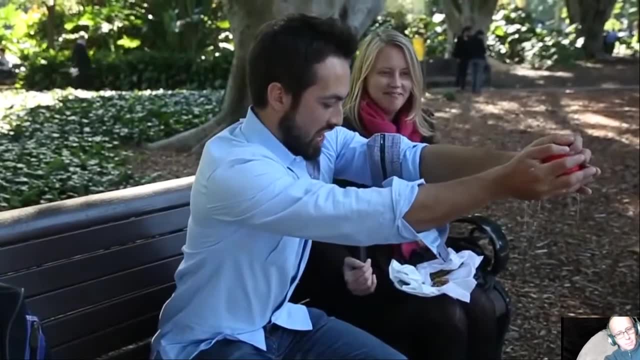 This is why it's so important that the sun's hot, because if the sun is hot enough, it gets these things moving so fast that sometimes they can't avoid a collision- Okay, And when they get too close they actually go An explosion. 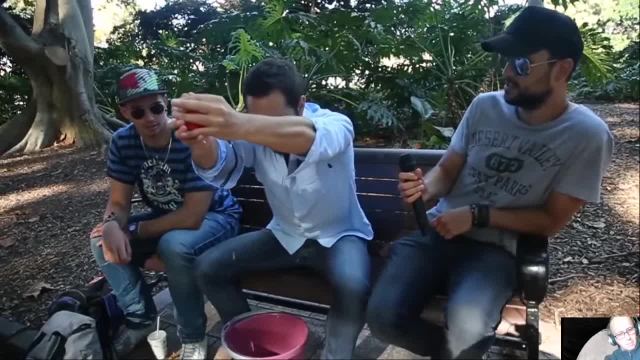 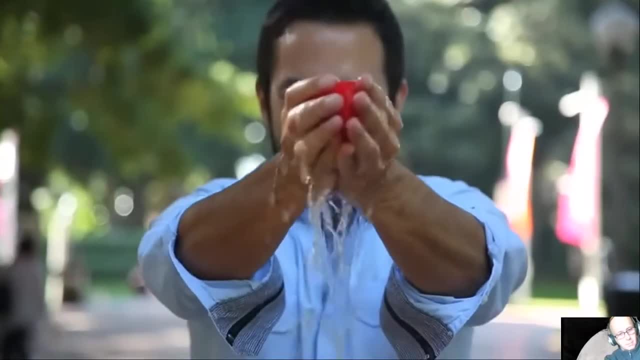 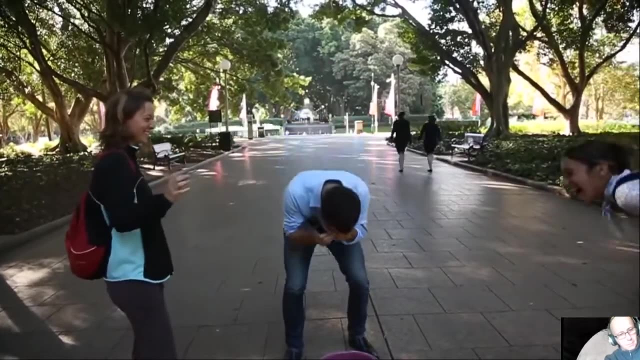 It goes everywhere. Wow, All right, Whoa, Whoa, Whoa, Whoa, Whoa, Whoa, Smash the protons. Yeah, yeah, yeah, yeah, No, no, no, Oh, And now they're stuck together. 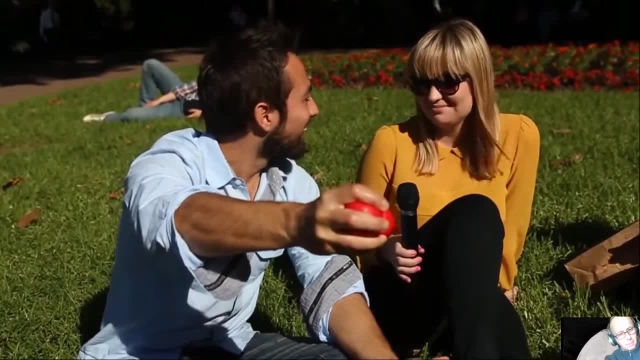 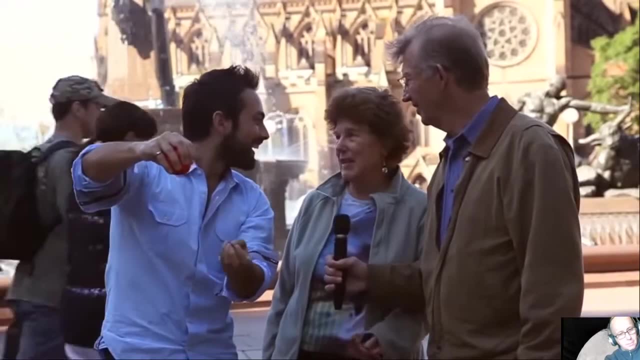 And you saw what happened when they smashed together. What happened? They leaked, They leaked, They leaked. Is that energy? Yeah, Sick. Well, the water poured out, but I guess energy would have poured out. The energy came out. 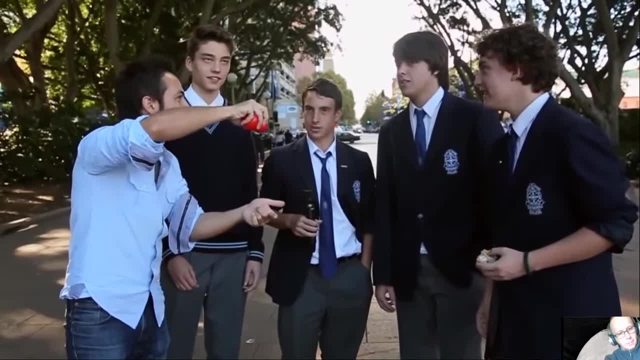 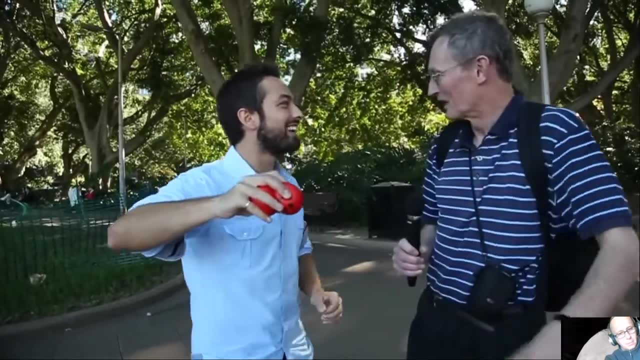 The energy came out. The energy came out. What was the energy before? it was energy, Stored energy, Stored energy. So what's happening there? It's releasing some mass by colliding, And that mass is Is converted into energy. It was the mass of the protons. 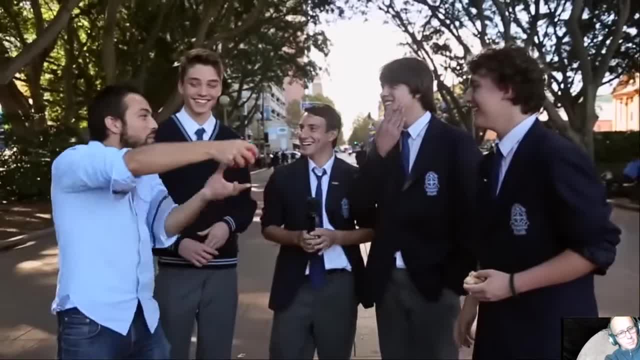 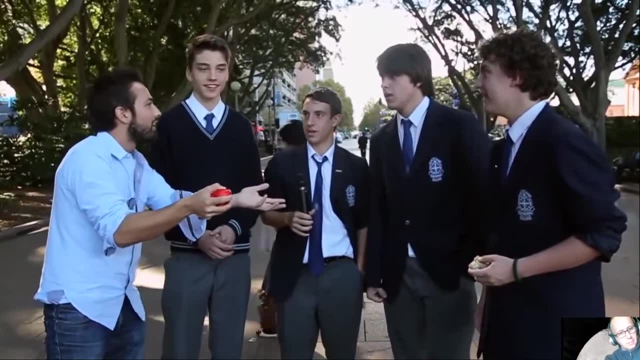 Oh, Oh man, When the protons smashed together, they got lighter. Yeah, yeah, yeah, And they lost that mass, and the mass was converted to energy. You know a famous equation about that: A equals mc squared. A equals mc squared. 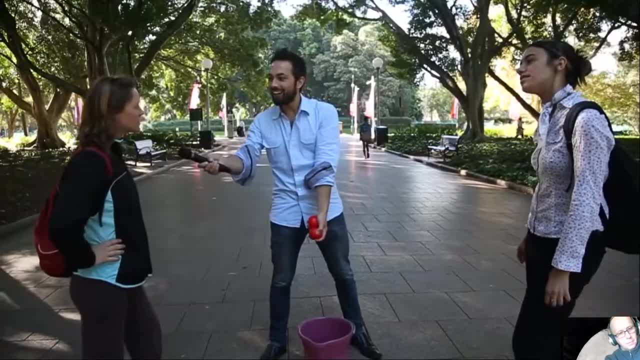 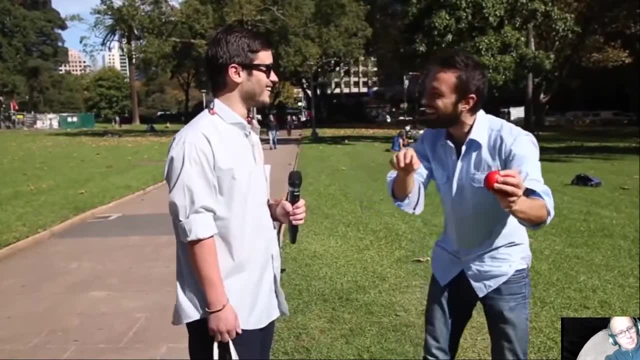 Yeah, A equals mc squared, E equals mc2.. Have you heard that famous equation Which, Which The protons and protons, makes energy? Well, A equals mc squared, yes. So what's E The sun? I don't know. 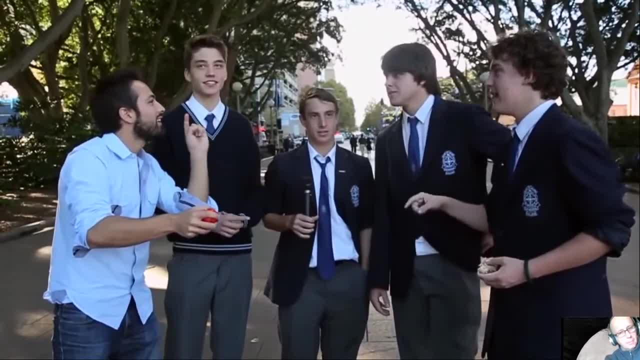 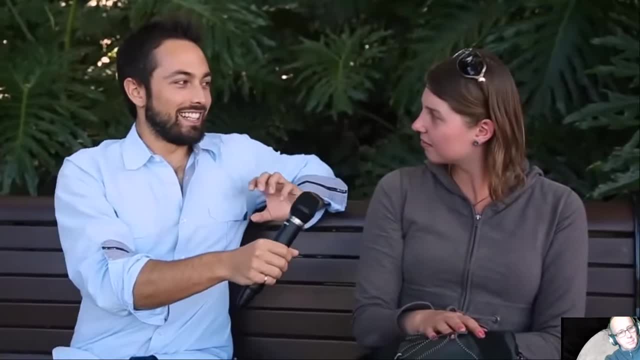 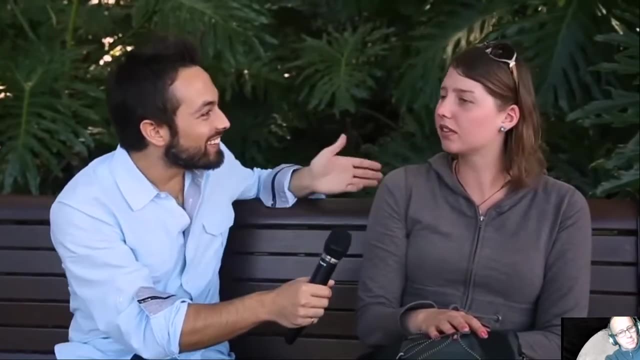 E is energy, M is mass Mass, C is Cassidy, Carbon. I don't remember what C means. So C is the speed of light. Speed of light, No, Really, Yeah, Oh, Isn't that weird, The speed of light. 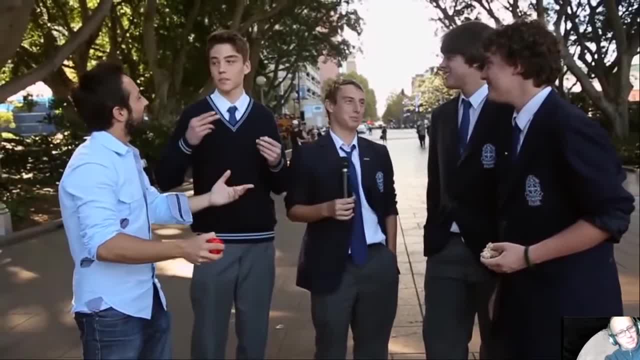 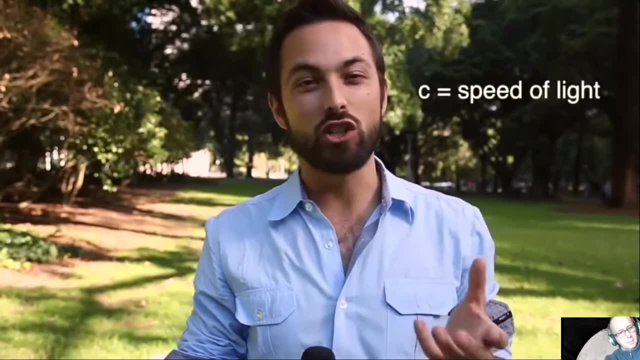 Right, Ah Wow, No wonder we dropped science. It seems most people have a tough time remembering that C is for the speed of light. Maybe that's because C is a bit of a strange letter to represent a speed. In fact, in Einstein's original paper he used the letter V for velocity of light. 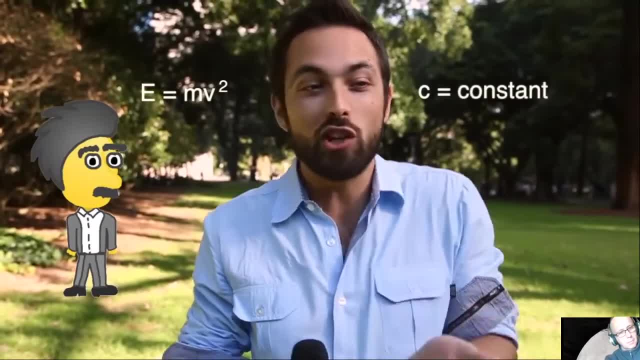 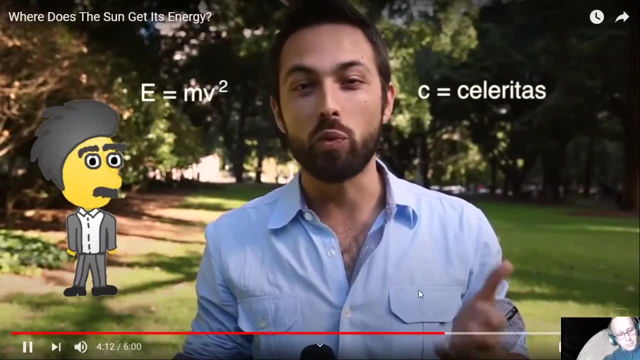 But nowadays everyone uses the letter C for constant. It's a constant of the universe: the speed of light, Though some people claim the letter C stands for celeritas, the Latin word for swiftness. What is that equation telling us about energy and mass? Energy equals constant mass. The mass and the energy combined together creates the energy. He's basically saying, like this mass that comes out gets converted to a lot of energy And the speed of light is a huge number. Yeah, If you think about that, a tiny bit of mass is a huge amount of energy. So every second, the sun is actually losing 4.3 billion kilograms Every second. Every second, That amount of mass is being converted into Energy. In the sun, hydrogen fuses together to form helium. But that's a little confusing, because how, out of only protons, do we create a helium nucleus which has two protons and two neutrons? 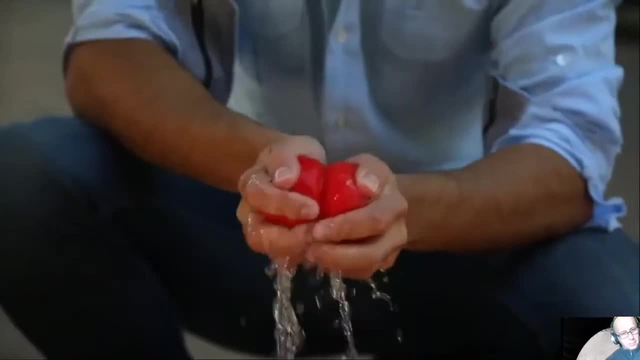 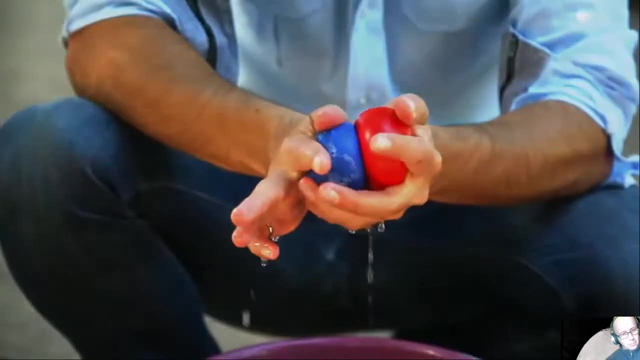 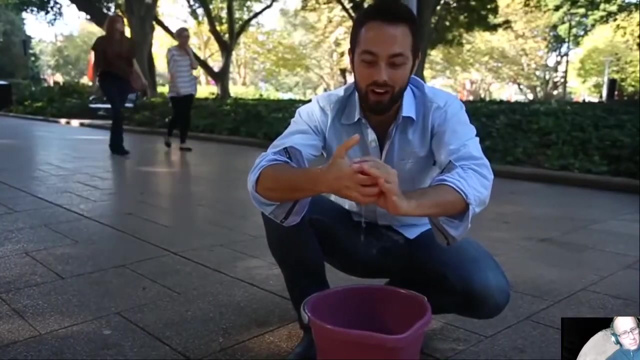 Well, the thing is, when the first two smash together, one of the protons actually emits a positron and a neutrino and quickly becomes a neutron. Next thing that happens is another proton smashes in And again we get more energy released. 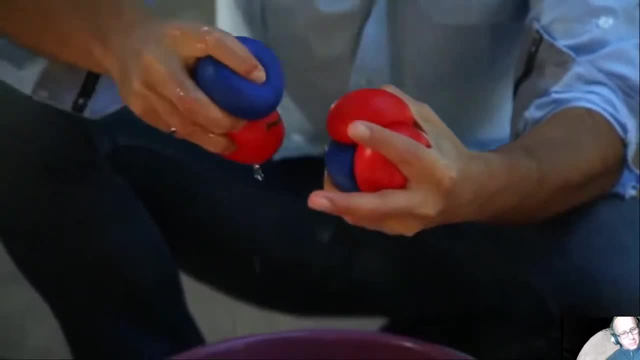 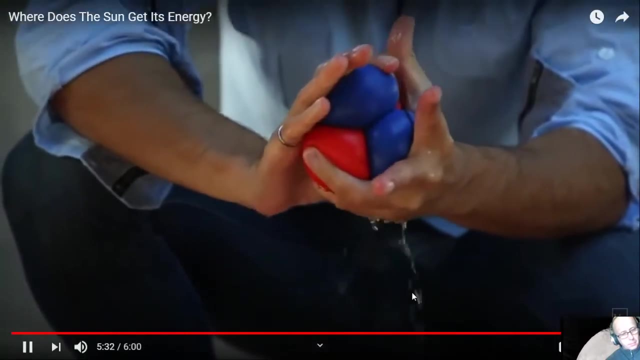 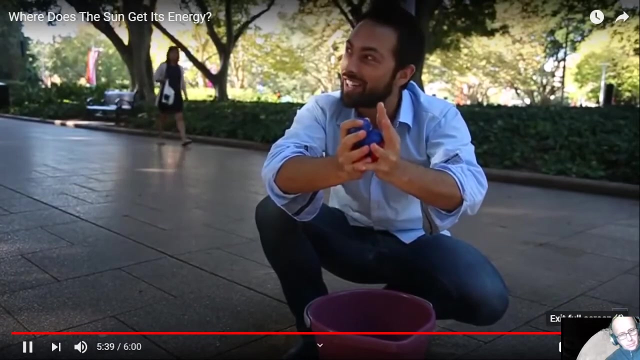 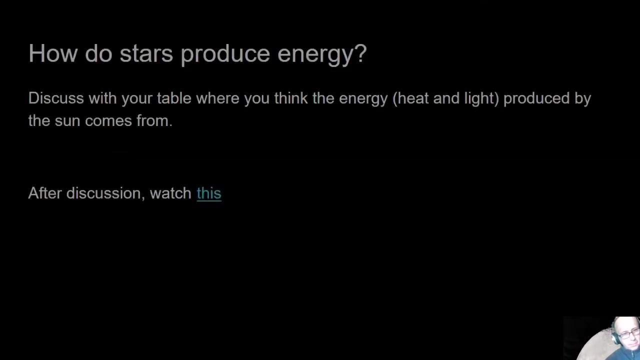 Now, if two particles like this collide, they emit two protons and what we're left with is the helium-4 nucleus. There you have hydrogen fused into helium And a lot of mass lost, a lot of energy released. If you want to know more about fusion in the sun, check out this. 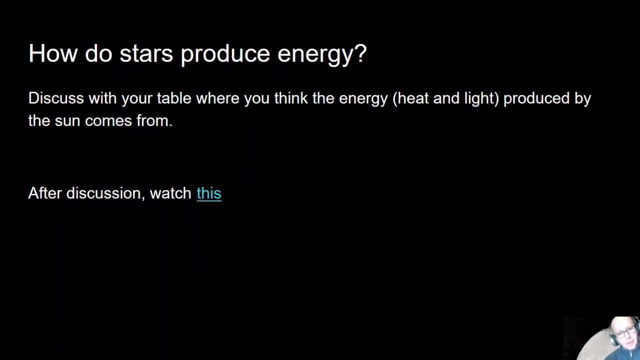 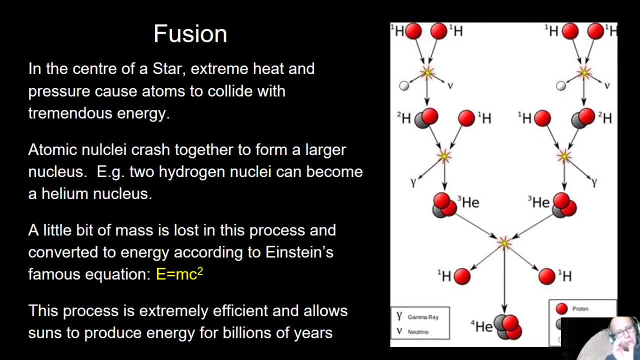 So I hope that's stopped the confusion about nuclear fusion. So this idea of nuclear fusion is the idea of hydrogen atoms fusing to make a larger element, which is helium, And from that we can actually make larger elements. So in the center of most stars you find hydrogen is actually fusing. 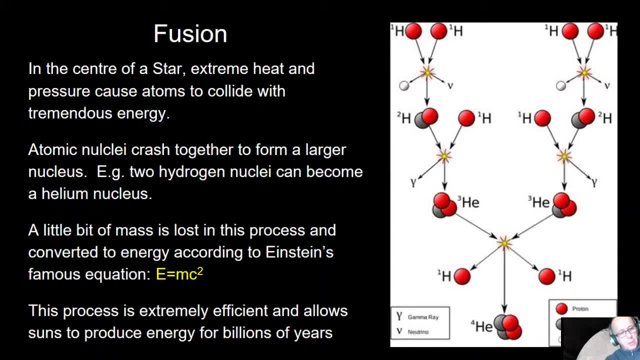 So the hydrogen can fuse to form a helium atom And this is explained by Einstein's theory of: E equals mc squared, where E is the energy emitted, mass is the mass lost and c relates to- I know it's confusing- the speed of light squared. 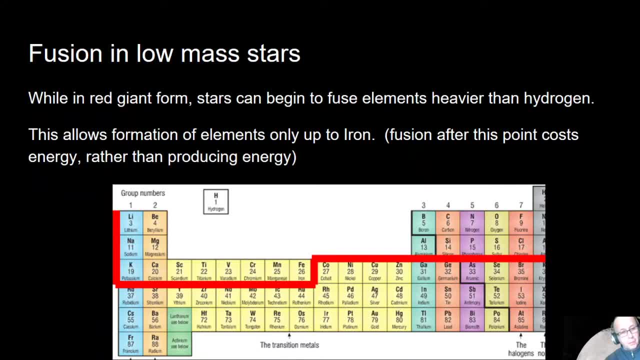 This process is extremely efficient. So, while in red giant form, stars can begin to fuse elements larger than hydrogen, So it has sufficient gravitational force that the nucleus can get close enough together for elements up to the size of iron Fusion. after this point costs energy. 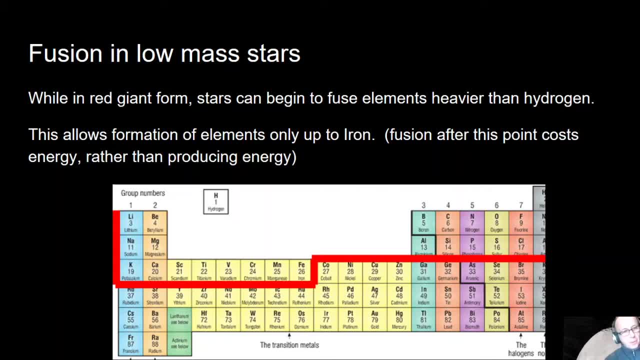 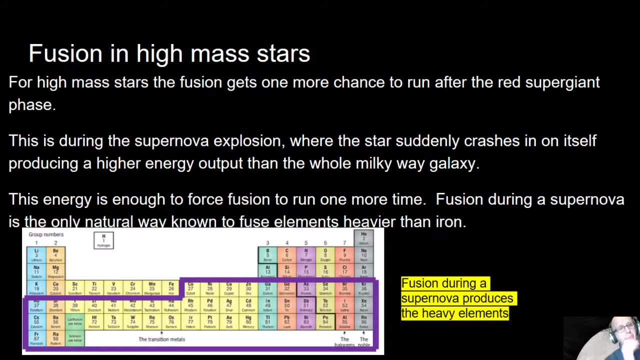 rather than producing energy. And for low mass stars that's as large as you can fuse when they're in red giant form. For high mass stars you can actually get to larger elements. So if they're up to the size of red supergiants, then you can make larger elements. 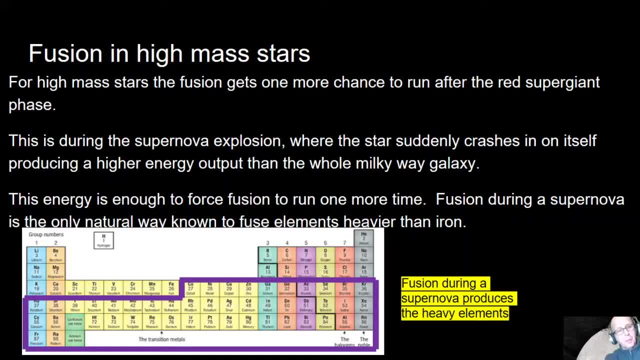 And this is during the supernova explosion, where the sun suddenly crashes into, where the stars suddenly crash into one another and you get high amounts of energy. So in supernova what that means is elements that are larger than number 26 on the periodic table can be formed. 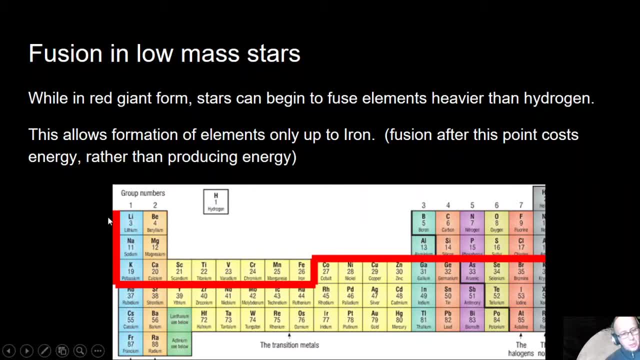 And that's the only place where they can be formed, Whereas in low mass stars this is as large as you can go. So the periodic table is based on the premise that we're going up in terms of atomic size. so how big they are. 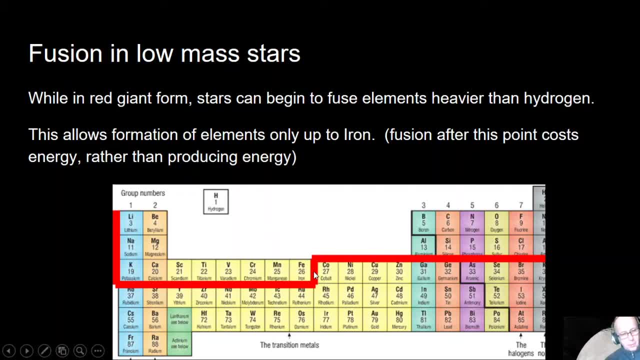 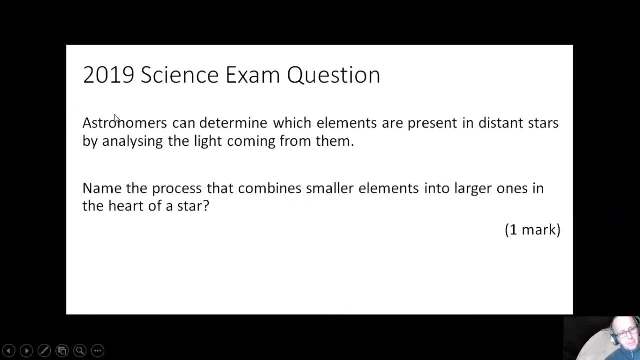 and 26 is the dividing line. Okay, so here's a question from the exam last year. Astronomers can determine which elements are present in distant stars by analyzing the light from them. Name the process. Hopefully you got that as nuclear fusion. 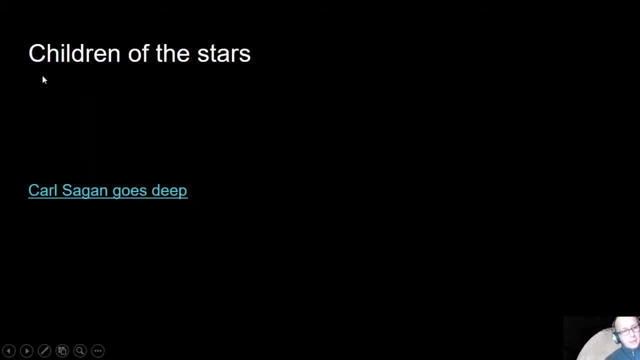 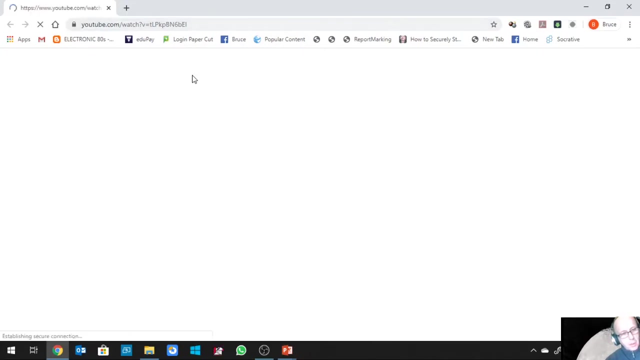 Let's stop the confusion, And this is a really good video to watch. It's Carl Sagan, who's a personal hero of mine. I'm just going to put it on towards the end so that you can have a look at it as well. 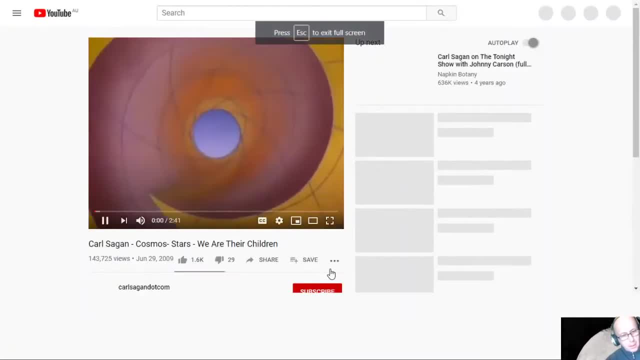 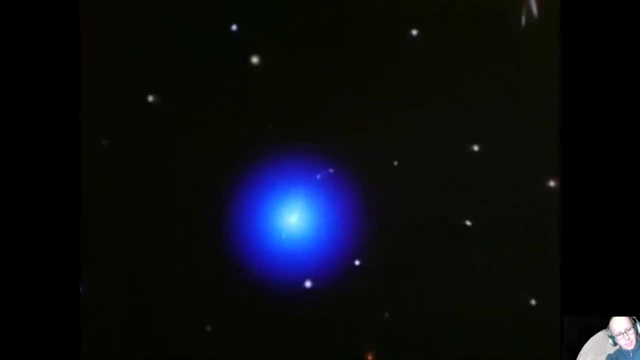 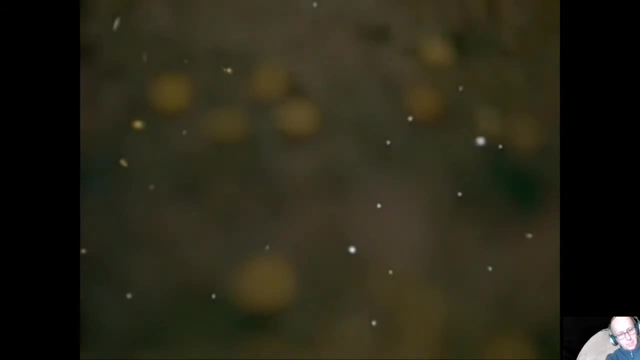 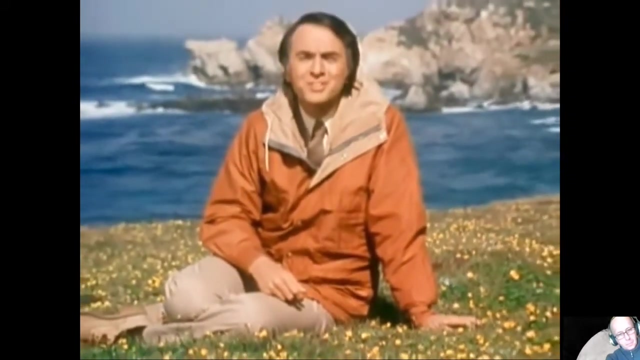 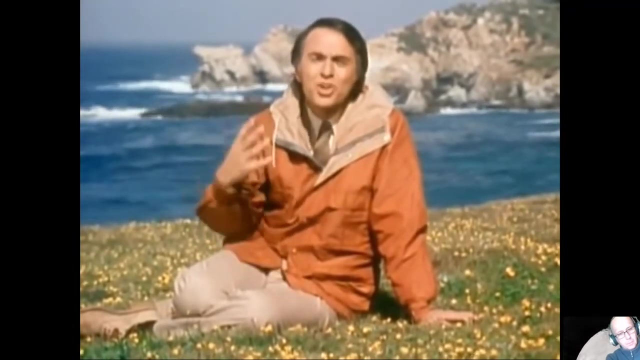 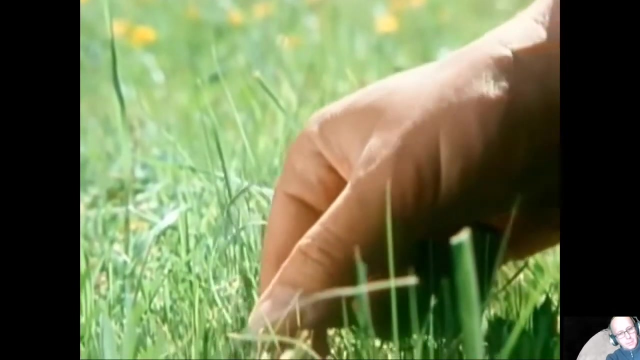 Okay. The lives and deaths of the stars seem impossibly remote from human experience, and yet were related in the most intimate way to their life cycles. The very matter that makes us up was generated long ago and far away in red giant stars. A blade of grass, as Walt Whitman said, is the journey work of the stars. 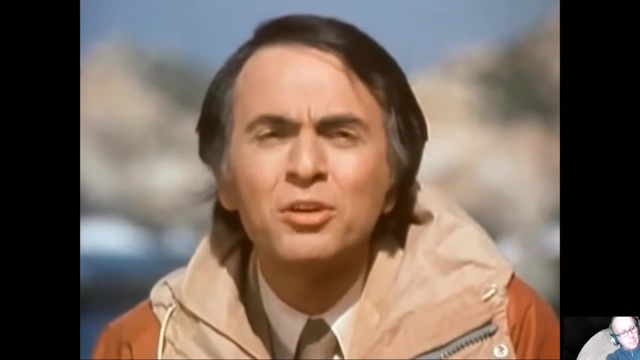 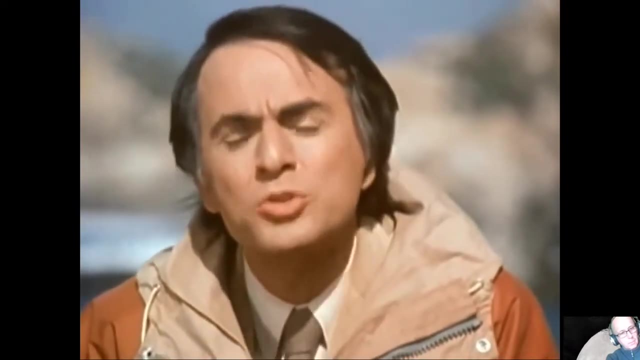 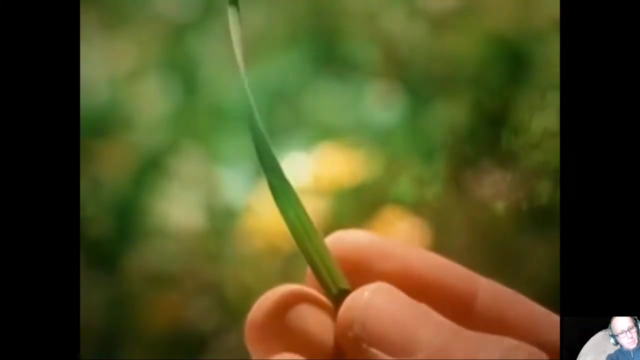 The formation of the solar system may have been triggered by a nearby supernova explosion. After the sun turned on, its ultraviolet light poured into our atmosphere. its warmth generated lightning, and these energy sources sparked the origin of life. Plants harvest sunlight, converting solar into chemical energy. 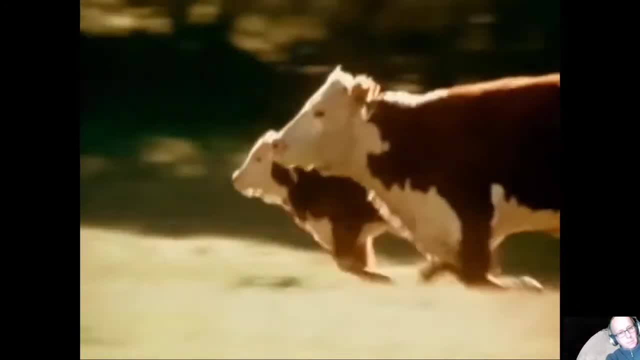 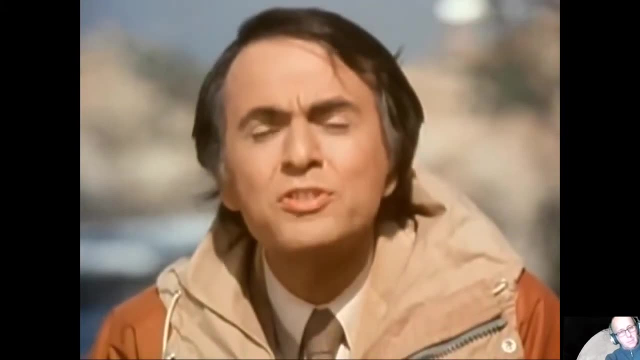 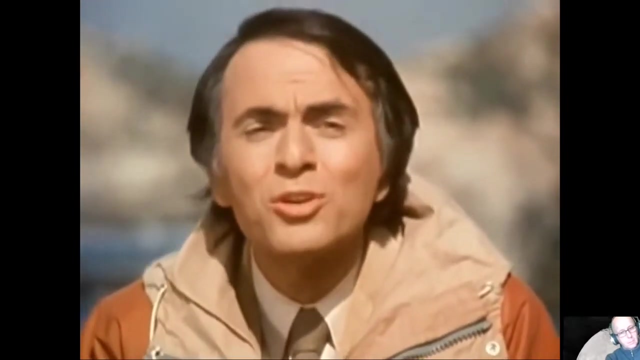 We and the other animals are parasites on the plants, so we are, all of us, solar-powered. The evolution of life is driven by mutations. They're caused partly by natural radioactivity and cosmic rays, but they're both generated in the spectacular deaths of massive stars thousands of light years distant.